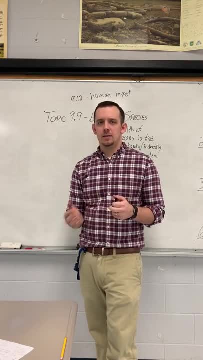 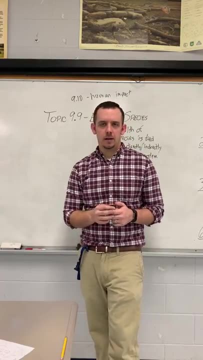 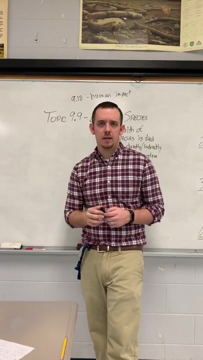 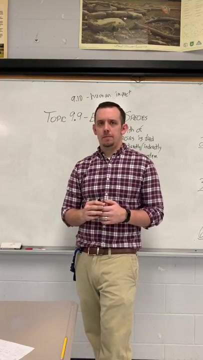 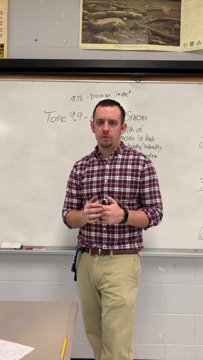 But the ideal behind this is that as I started looking at the curriculum, I became a little paranoid that I wasn't going to be able to cover all the topics in class. Okay, so I'm still working down the progression of topics that we covered in the class my first year teaching the class. The next year I'll obviously plan better But moving forward, rather than cram everything into the remaining four months that we have in class or four months we have before the test, I was going to start at the bottom or the last topic and work up. 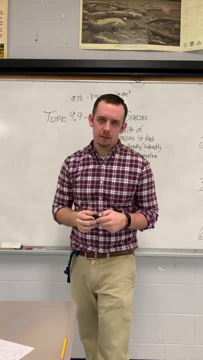 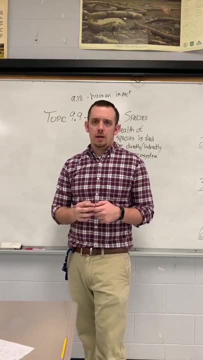 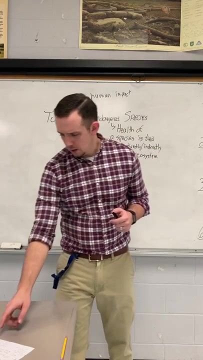 Okay, meet in the middle or maybe I get to the topics in class. Like I told one of my corresponding teachers, at the least they would be review videos for my students. I'd like to give a shout out to Mr Warczyk on our National Apes group on. 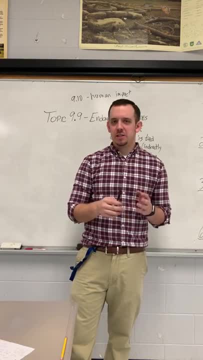 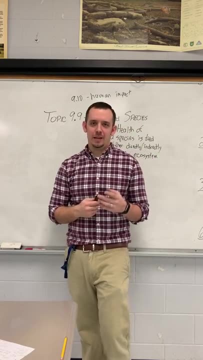 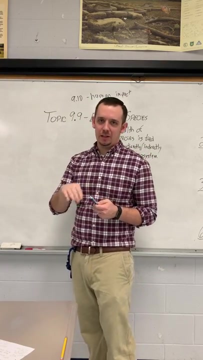 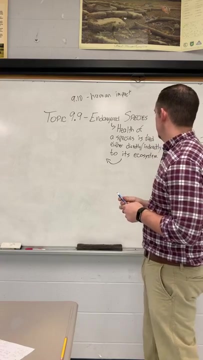 Facebook. He recommended adjusting my videos or my filming to make it more eye level, so that's why you're seeing me kind of more at a level distance rather than me looking down at the phone. Okay, without further ado, let's get started on topic 9.9: endangered species. When we think about endangered species, I 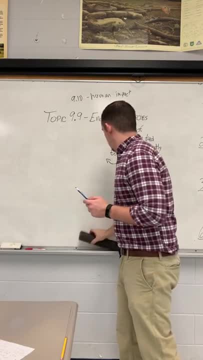 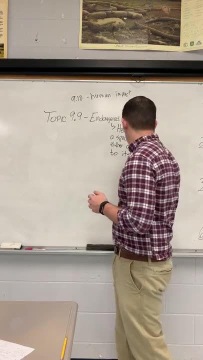 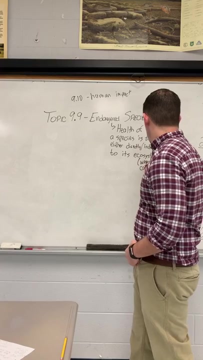 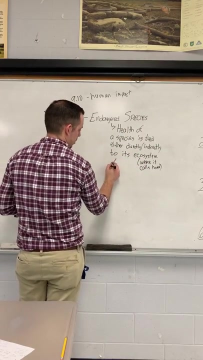 want us to think. this little statement: The health of a species is tied either directly or indirectly to its ecosystem, And by ecosystem just think of where it calls home or its habitat. Okay, all right. and as a result, changes to that ecosystem, minor or major, so they can be small or big changes. 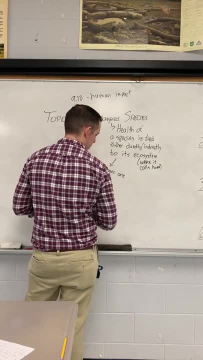 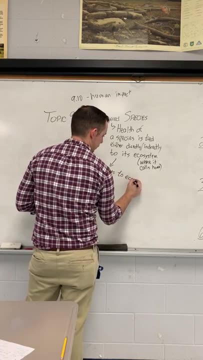 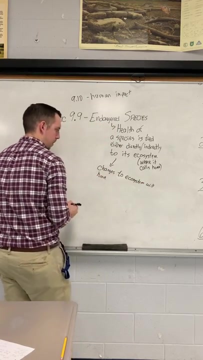 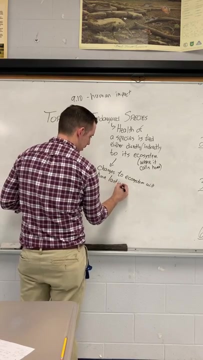 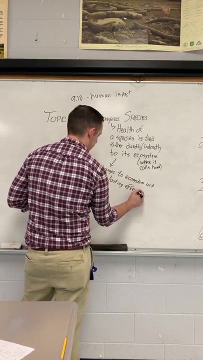 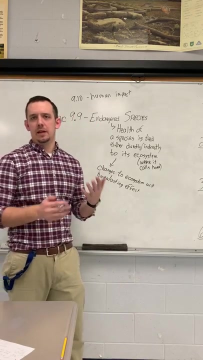 Okay. Or changes to ecosystem will have a lasting effect. It'll have a. it'll have consequences. There will be consequences to any of these changes. Have a lasting effect, All right. so I was thinking about this and I think about it, as with humans, we 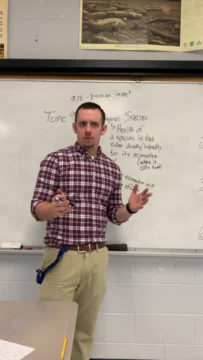 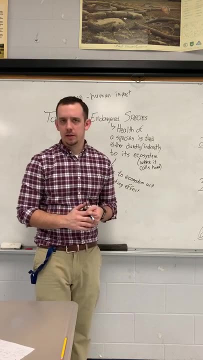 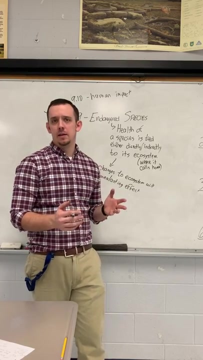 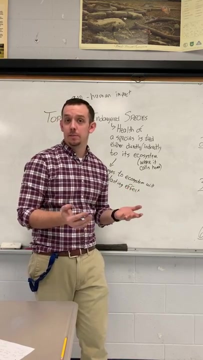 all- excuse me- we all either rent or buy a home, but regardless, we all are invested somewhat into a living space or to into a home. If something happened to that home, it could be the electricity goes out. That's that. that's a minor change. to some it's a 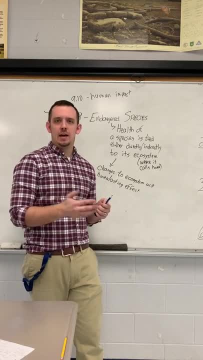 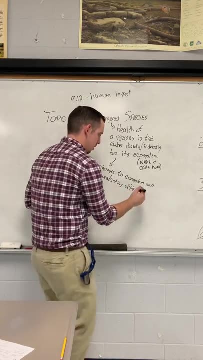 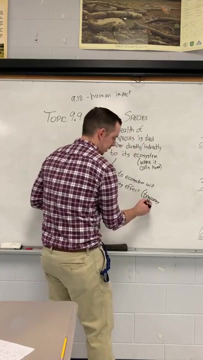 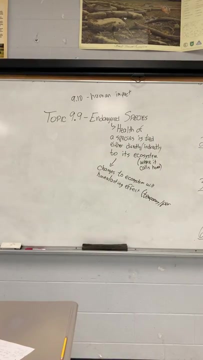 major change to others, but that change is going to have a lasting impact. Okay, it's going to have a lasting effect. It could be temporary. so it could be temporary, as the power outage would be, or it could be more permanent. Let me make sure we can. we can get everything right on the board, Okay. 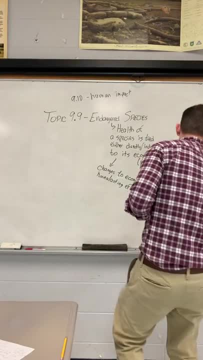 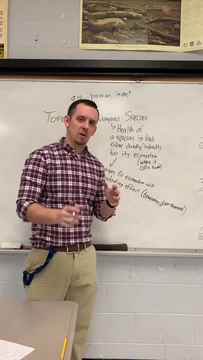 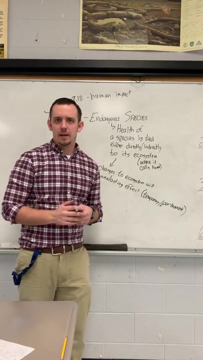 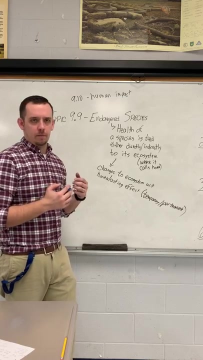 Or it could be more permanent. for instance, someone's home burning down, That's gonna have more of a long-term effect. or compared to the power outage, okay, We are invested in that home. If something happens, a change to that home, then we are going to- we're going to feel the impact of it. Okay, it's not directly impacting. 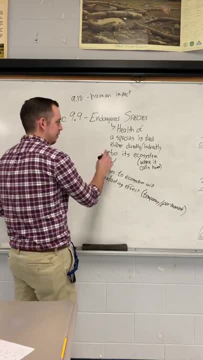 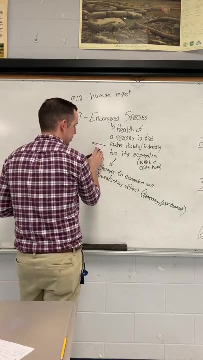 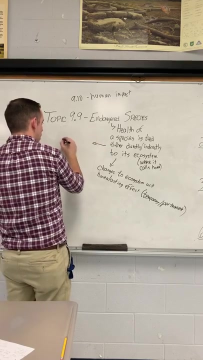 us, But still that is our okay. the same is true with nature and animals in the wild, All right, so these could some examples or factors that could lead to the health of the species are related to temperature changes, So these are gonna be changes over here or factors. 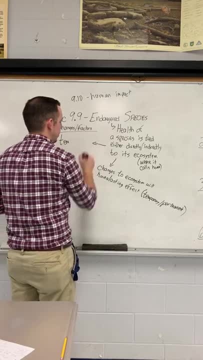 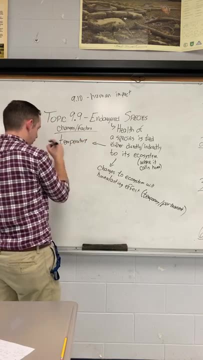 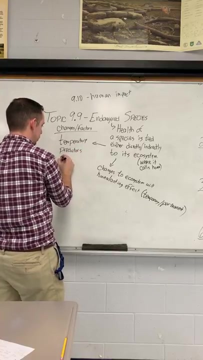 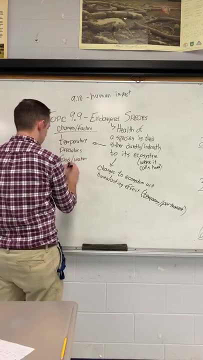 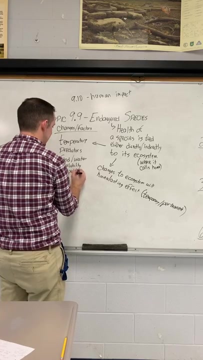 Factors that we have to consider that are gonna play a role on these endangered species, So temperature predators, other resources like food, water availability- And I would throw competition in here as well, Because as these others become more scarce, the competition will be lower. 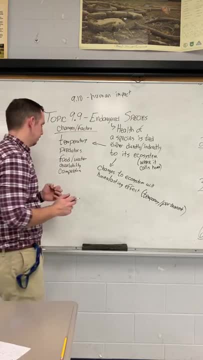 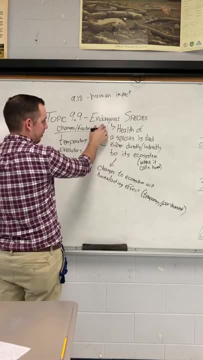 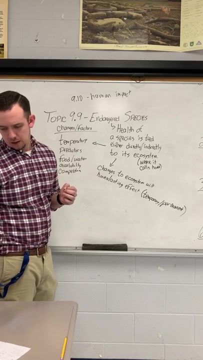 So the competition is going to increase, all right. So these are changes and these are changes to the ecosystem that are gonna have a impact on the health. all right, If these factors occur. so if the temperature changes, if there's an increase in predators, 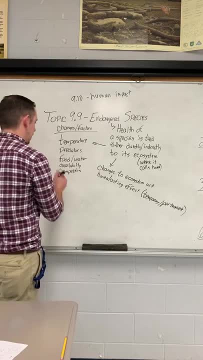 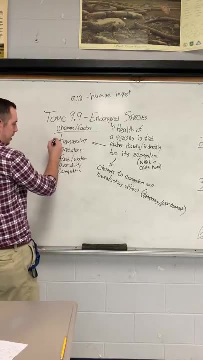 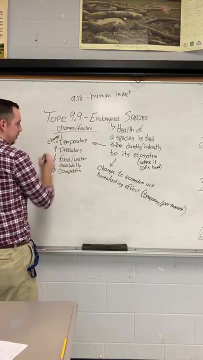 if there's a decline in food. so decline in food, increase in predators, increase in competition, I'll just say change, it could be an increase or it could be a decrease, depending on the habitat. Change in temperature Then, and we'll draw my arrows to, so we're connecting. 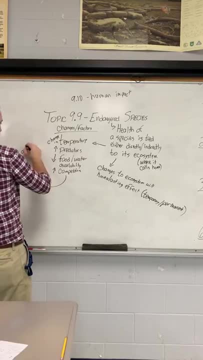 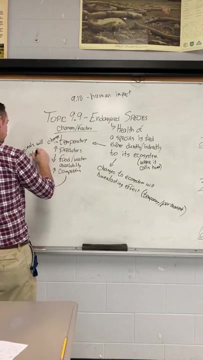 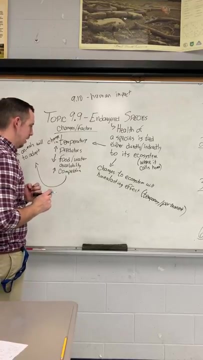 Then animals, because we're gonna be referring to immigration here, immigration with an E, Then animals. we'll need to adapt, okay. So adapt to these changes If there's an increase, I'm sorry if there's a decrease in food and water available. 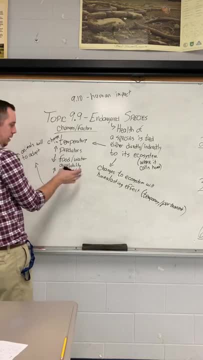 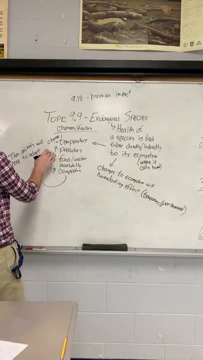 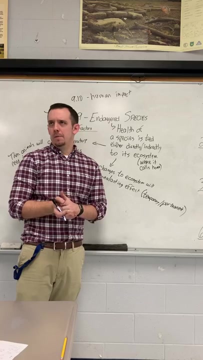 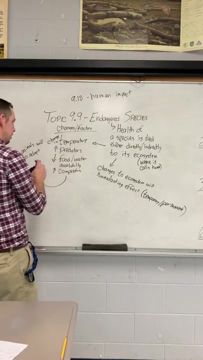 they're gonna have to adapt and either find something else to eat or, unfortunately, unfortunately- die out. There's an increase in predators, some things that they would have to adapt- maybe some chemicals, Some camouflage adaptations, Some defense mechanism adaptations- So there would have to be some adaptations take place. 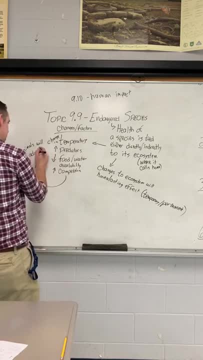 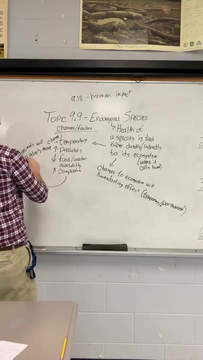 as a result of these changes. So they would have to adapt, move or immigrate out out of the area, So they'd have to find somewhere else to live Or, unfortunately, they would die. okay, And that's where we get this endangered species. 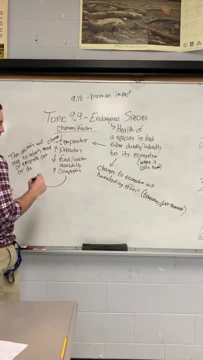 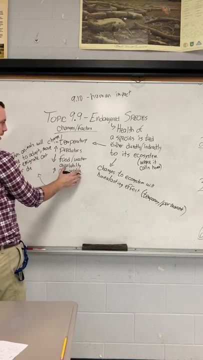 So three things would have to happen if these changes or factors take place that are going to hinder the survival of the animal. They're gonna have to adapt. that's number one. They're gonna have to adapt. They're gonna have to immigrate or exit the area. 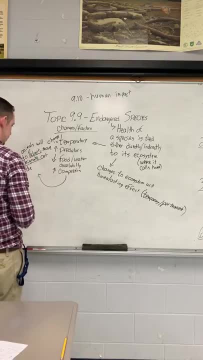 That's where I tell my students to remember that immigrated versus immigrate with an I is this immigrated is exiting or they would die out. okay, I'll pause, or I won't pause the video, but I'll step aside And you can pause the video to. 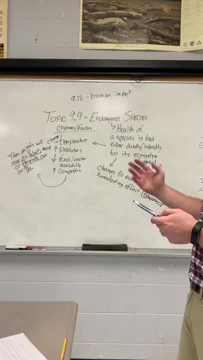 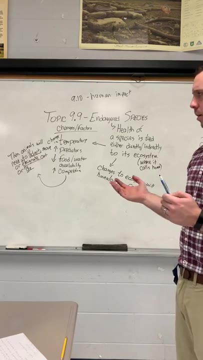 write down the notes from the board. And again I told my students I'm gonna do it. okay, my students, I'm treating this like a lecture that I would give them in class. okay, so of course, in class I would have interactions and discussions with 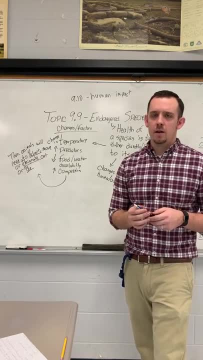 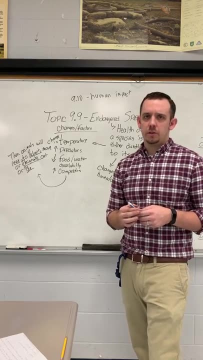 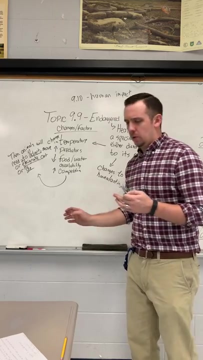 students, but obviously we can't do that via YouTube. of course, you could ask questions in the comments section and I could answer those questions, but I wanted to present it like a lecture. okay, so I'll talk to my kids, I write notes on the board, I step aside and I'll let them copy down their notes while we are. 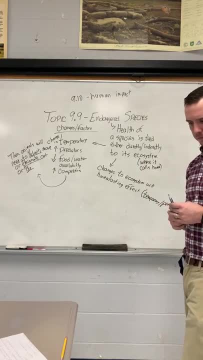 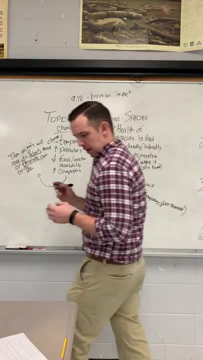 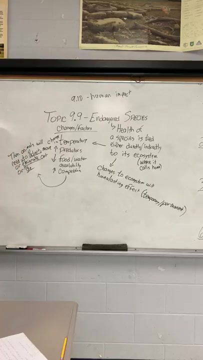 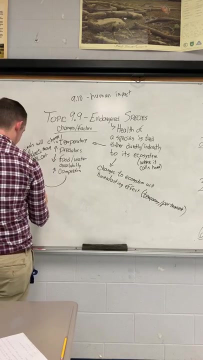 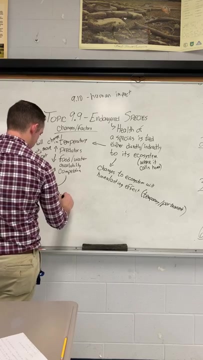 still discussing. okay, all right, this last point that I wanted to make. I don't want to erase anything because might be some stragglers coming in late. our solution is selective pressures, so these are going to be more specific pressures that are going to affect the. 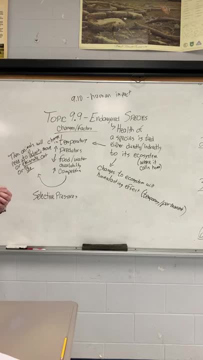 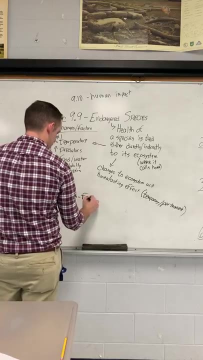 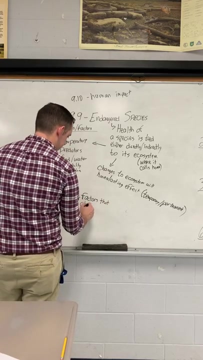 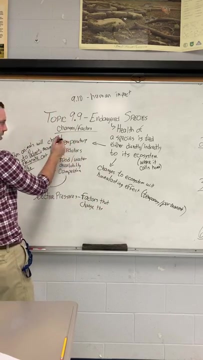 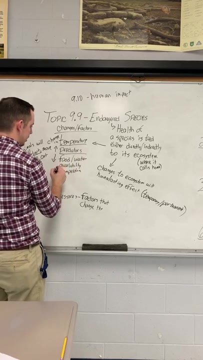 the well-being of the species. okay, and selective pressures are factors that change the behavior of a species. okay, so these could be the same factors that we've already mentioned. so we have temperature, and I'll underline these: temperature increase in predators, decrease in food and water availability, increase the competition, so these could. 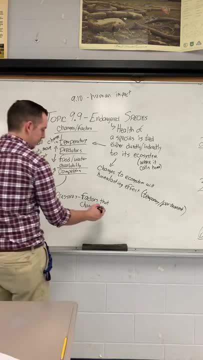 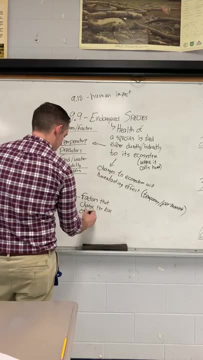 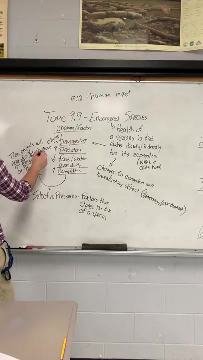 be selective pressures as well, but these are going to change the behavior of a species. okay, so this will be cheap insight. Grab your that. you're already got ahadau inward selectors. emotionallyminimally you're going to get easier to fit the. okay. so this will be timing and we are this adaptation. if I want a connect, my 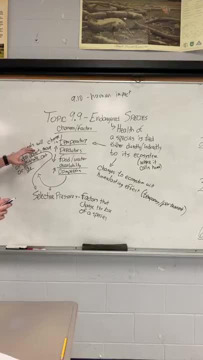 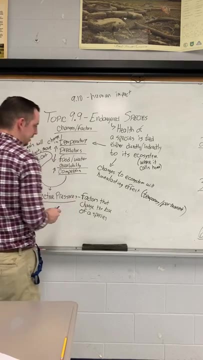 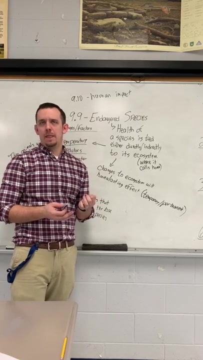 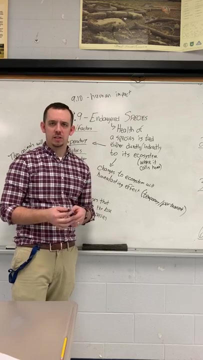 adaptation with a select pressures and realize this might be a little bit confusing as far as the organization and I'll try to clear it up by the end of it. okay, so a species may become more aggressive, it may become less aggressive, they may become more, more of movers versus a more lethargic style. okay, so they may have to understand that in order for 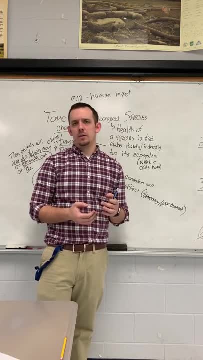 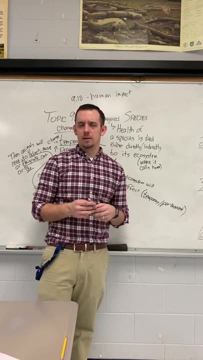 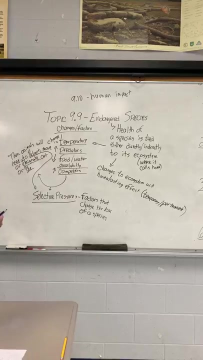 my survival. i need to figure out, or i need to adapt to climbing trees versus hanging out down here in the amongst the flowers if i want to survive. okay, so these are called selector pressures. all right, so this is really the meat of this unit. okay, so this unit of endangered species? 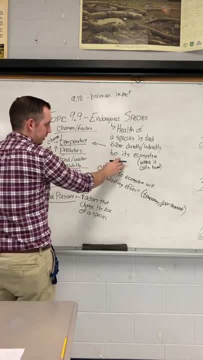 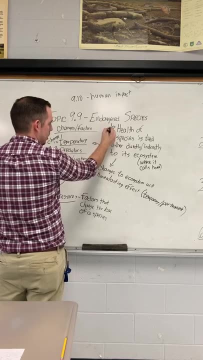 health of the species is tied either directly or indirectly to its ecosystem. how changes to that ecosystem will have a lasting effect on the environment, and the environment will have a lasting effect on the environment, and the environment will have a lasting effect on the environment effect. okay, so we got this point first: how changes to that ecosystem will have a lasting effect. 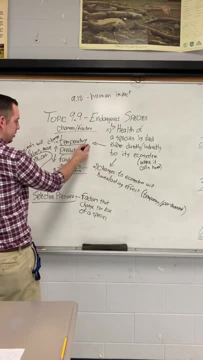 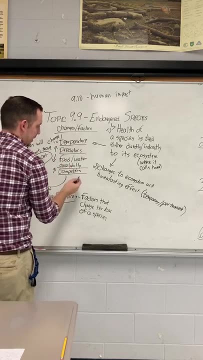 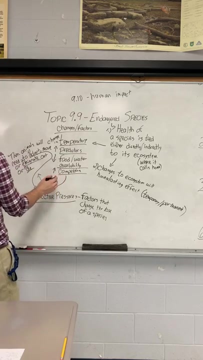 what are those changes? okay, those could be temperature changes. uh, those could be an increase in predators, there could be a decrease in the resources we have available, or there could be an increase in competition, which is tied in with these other two. okay, um, examples of this, i'm sorry, added on to this, factors are: 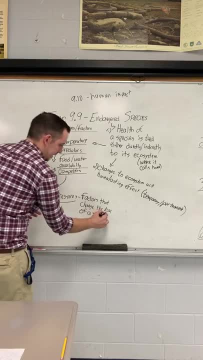 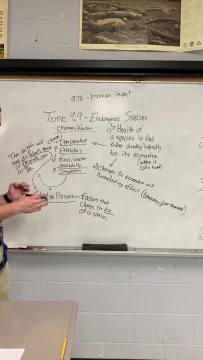 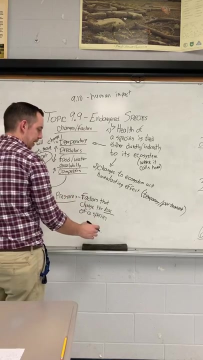 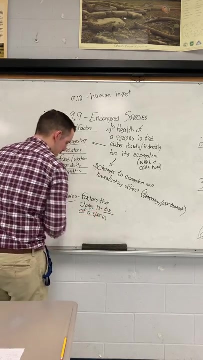 selective pressures which specifically change the behavior. okay, so we're not talking about the food and water that an animal needs to survive, but more so how that animal receives that food or goes about obtaining that food. okay, so this is more behavior related. now i wrote bx. my students understand bx is. 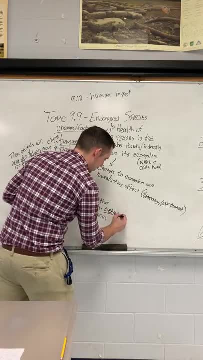 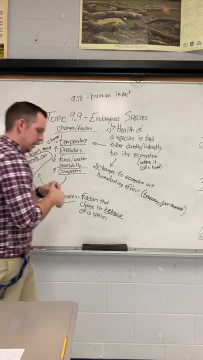 okay, so this is more behavior related. now i wrote bx. my students understand bx is better behavior, but some of you may not know that. uh understand that. so that's changed the behavior of a species. all right, let me see how much room i have on the left side of my board. 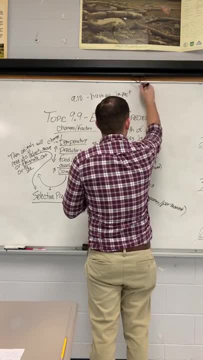 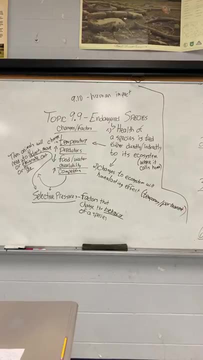 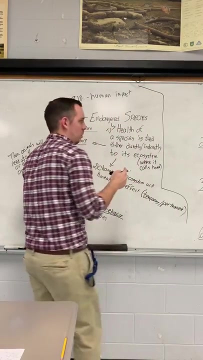 not a lot, so i'm going to write, box off this and try to fit. like i said, i don't want to erase any of my content on my board. yeah, i should have enough, all right, um, so what? what can we do? these are all problems, and this is obviously not a good thing. we, as 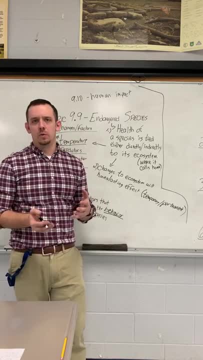 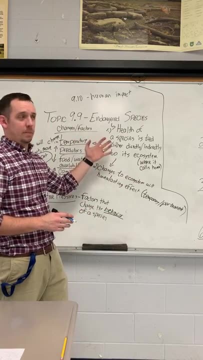 students of in the environment or students that want to focus on preserving the environment need to know: yeah, this is all not good, this is a bad thing. what can we do to fix it? okay, that's what i'm going to talk about next. all right, so what? 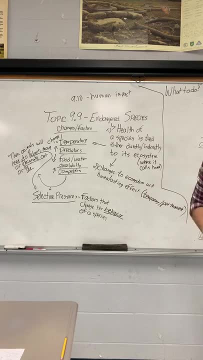 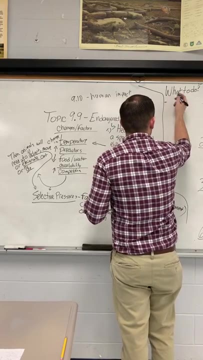 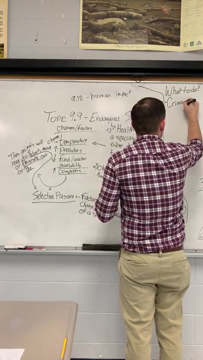 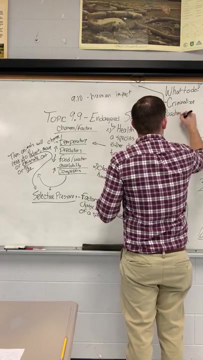 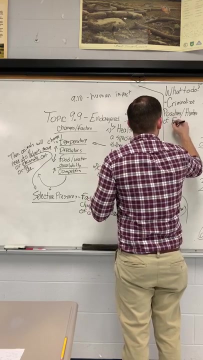 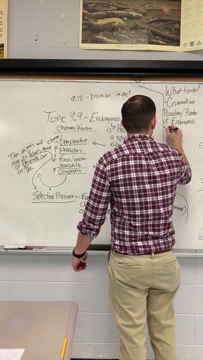 to do, make sure my, all my, and i'll just write under: yeah, we can see that. what to do, all right, so some things that, um, that we can do to solve this problem. um, we can criminalize, uh, poachers, hunters of endangered species. we have these all over the world, poachers, vicious men and women who 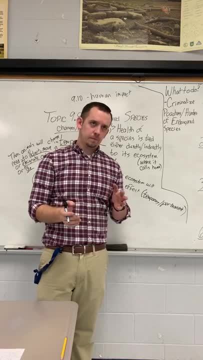 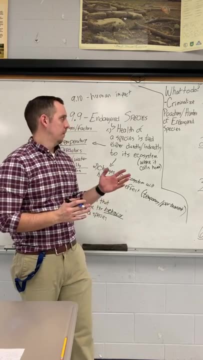 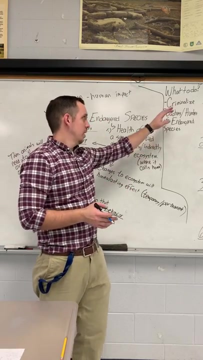 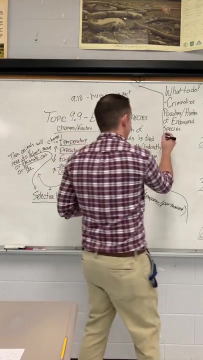 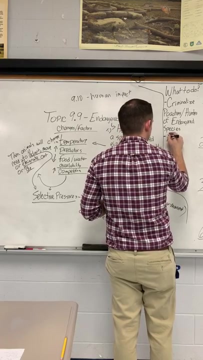 are hunting down these animals, whether it be for material gain or what have you, and they're killing these animals that are already at risk. okay, so that's one thing that we could do is increase the penalty for those behaviors, all right. another thing is: we could start more, so we could establish. 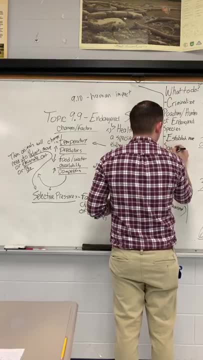 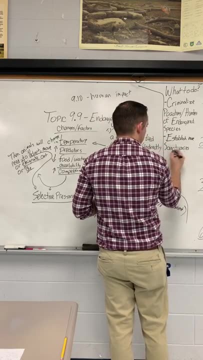 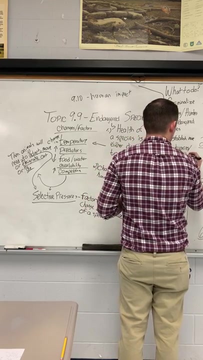 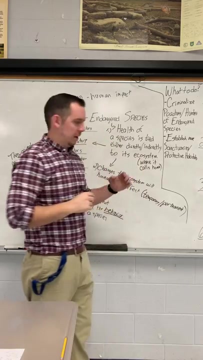 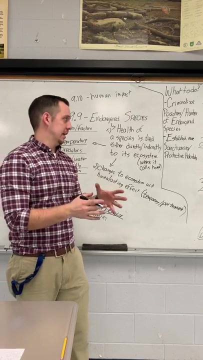 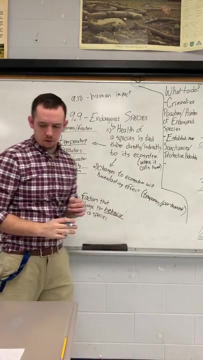 more sanctuaries, more protective habitats for these animals. sanctuaries, um, i'll just say protective habitats, okay. so if they're already endangered, if we can, if we can all keep them all in a safer environment than the one they're already in, than the one that's causing these stressors on their planet. 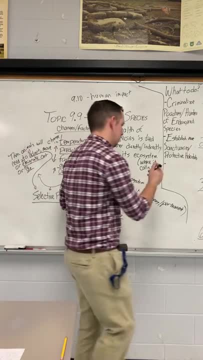 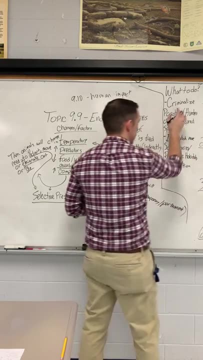 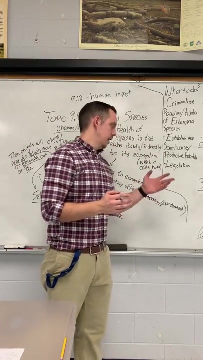 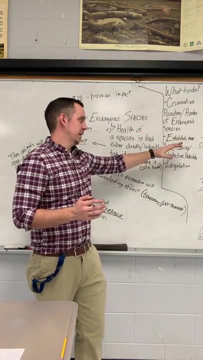 lives okay. And then, lastly, is legislation Okay. so this is tied in with this first one I mentioned about and, as well as the second one, We could talk to our legislators about implementing some of these laws to criminalize poachers. We 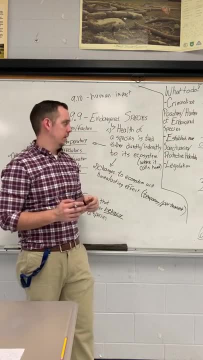 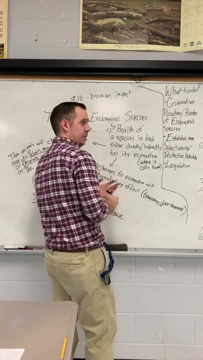 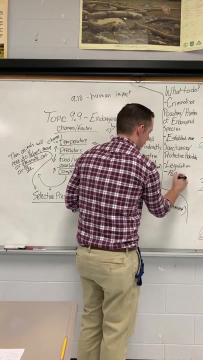 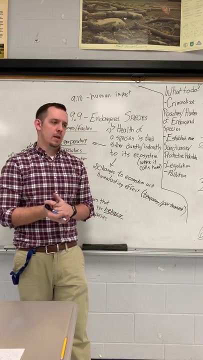 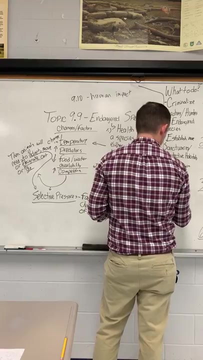 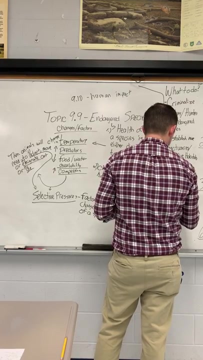 could talk about. we could talk to our legislation about more sanctuaries, more habitats, more protective habitats. some other ideas that I've thought about: More pollution laws- I mean pollution is eliminating animals daily. More environmental friendly- so environmental friendly- laws, For example, our state parks and our national. 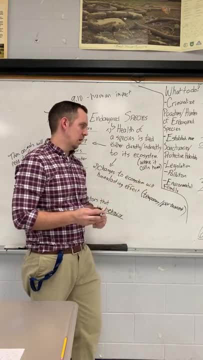 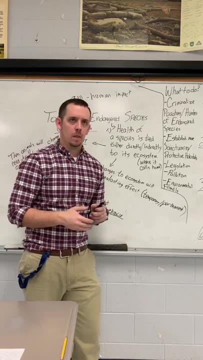 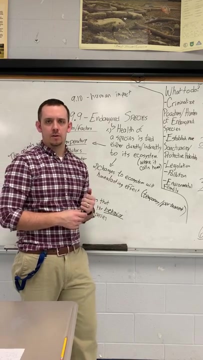 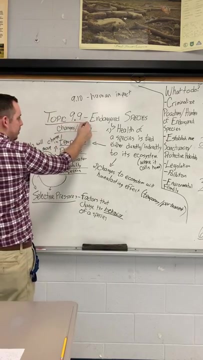 parks established, talked to our legislation about establishing more laws in those particular areas to protect our endangered animals. Otherwise, we may have it, we may see an increase in the number of endangered species that we have currently. Okay, so this was 9.9, topic 9.9 of our AP: environmental endangered species. Thank, 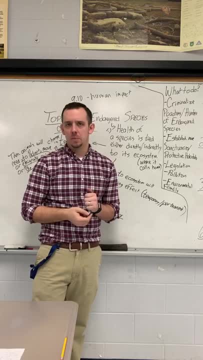 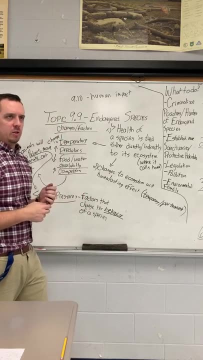 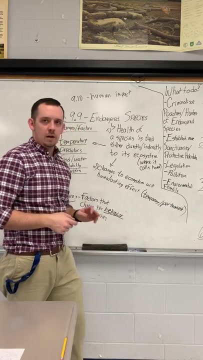 you again for tuning in. Hope you check me out next time on topic 9.8.. I'm not sure when I'll get to that video, but I'll get to it as soon as possible. Okay, thanks again for watching the video and hope you subscribe and hope to see you next time. Bye. See you next time.